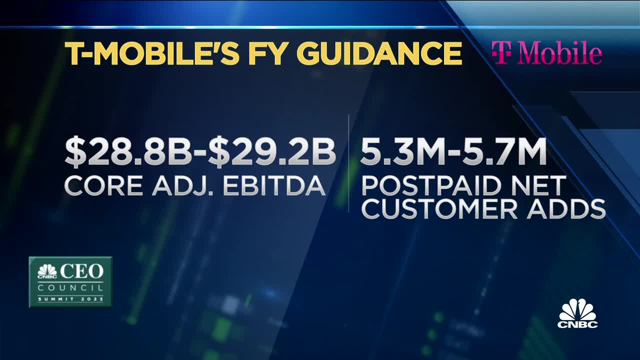 And look you compare cash flows in this industry- I won't talk about T-Mobile. Cash flows in our industry are double what they were in 2014 during the 4G era, And yet the consumer is getting four times more for their dollar. 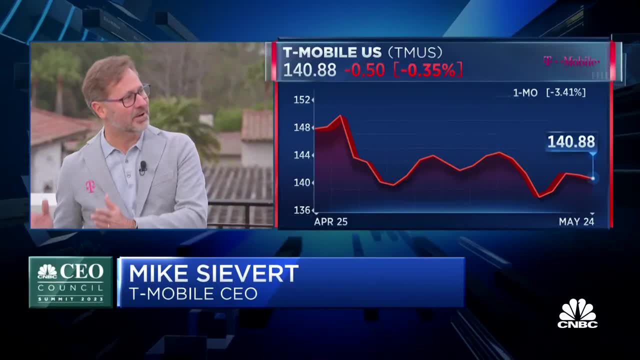 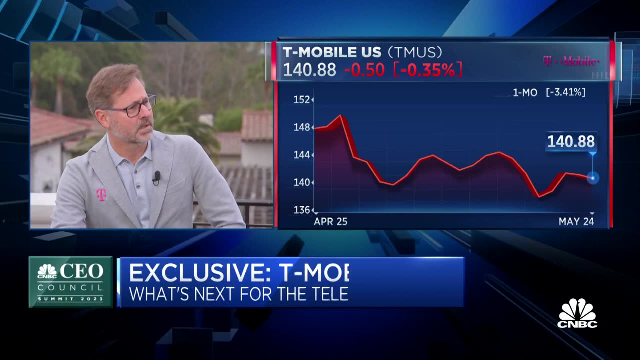 So how could that be? How could the consumer be winning? and the category winning It's 5G, That's the 5G dividend. And so you know this is a healthy, vibrant sector, But isn't cable now taking half of the industry? ads. 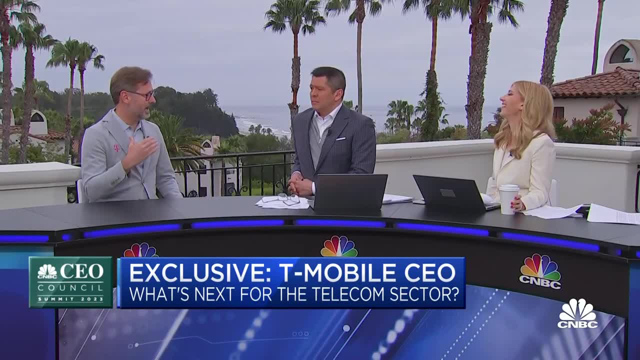 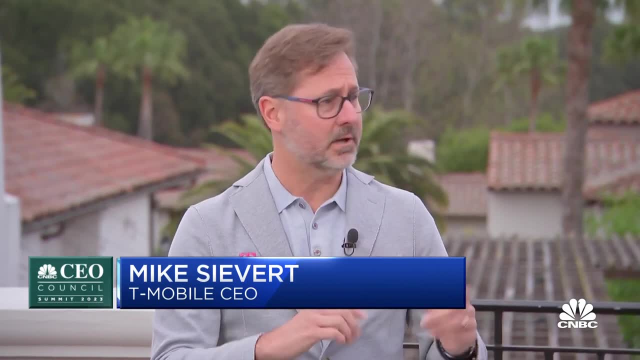 Well, you know, look, I mean again- we guided up our net ads this quarter after outperforming expectations, And so you know, yeah, there's a dynamic going on there that may be hurting some of the others. On the other hand, they're monetizing that relationship as a wholesale provider. 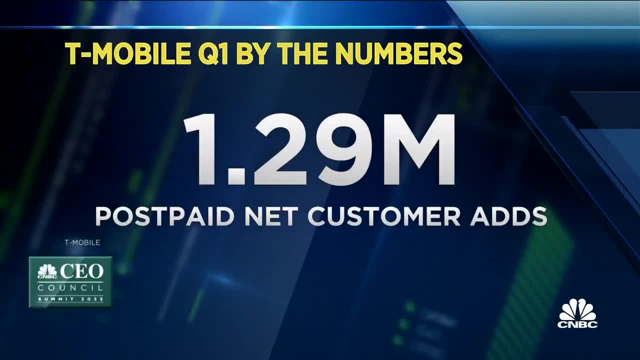 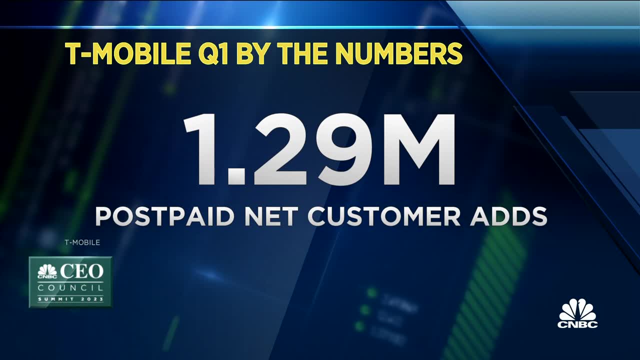 And so they have other ways to make money. You know cable's growth is higher than a year ago, But as it relates to us, our porting ratios versus cable have been better versus a year ago for five straight quarters now. So it's just not coming from us. 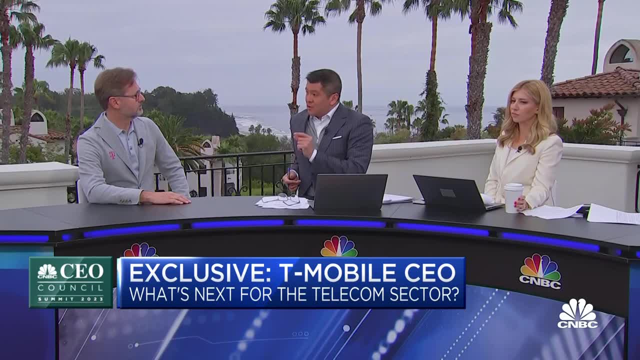 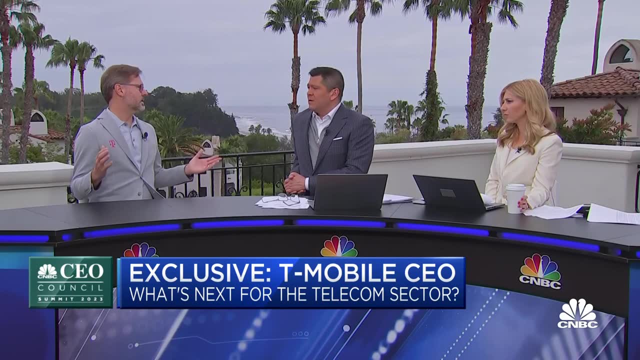 But if there's incremental scarcity with a more discerning consumer, do marketing wars heat up here? I mean, do people start getting really serious about outreach? Well, marketing wars have always been heated up. But to the premise of your question, that plays to our strength. 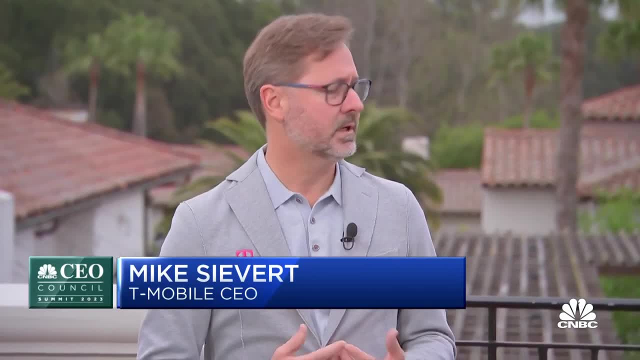 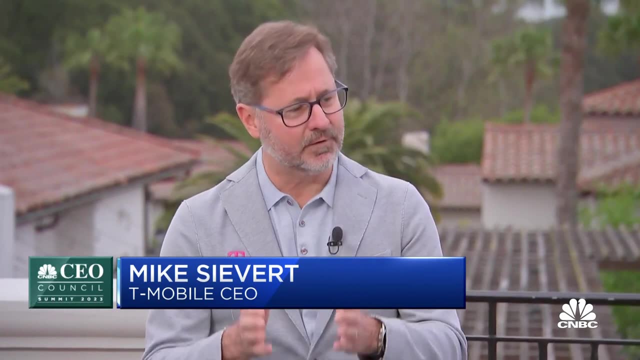 If the customer becomes more discerning. that's good for T-Mobile. You know we've always been the value leader. That's important in a time of, you know, questionable economy. But at the same time now, for the first time in our history, we're the network leader. 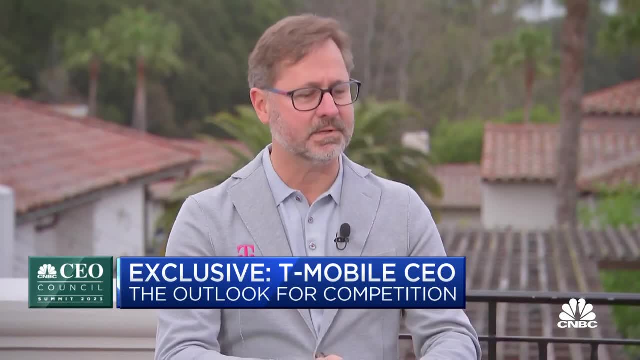 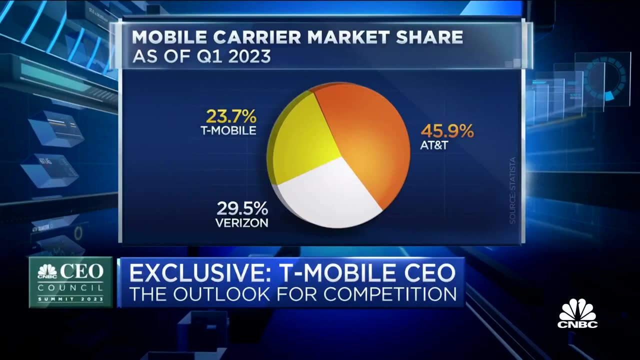 And that's the promise we made. You know I've talked about that before here. We wanted to be simultaneously the network and the value leader, And now we are. And so what's happening is now tens of millions of people, prime credit customers, the best paying customers in the industry- are looking at T-Mobile because we have the strongest network. 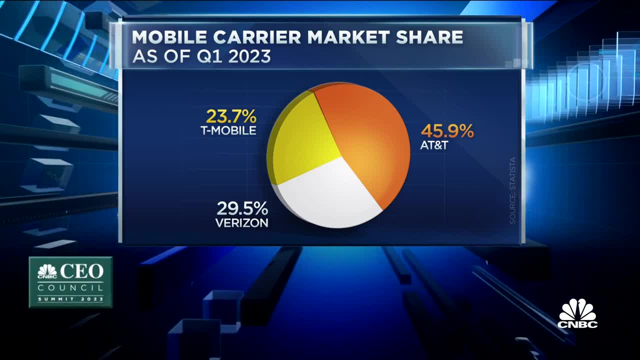 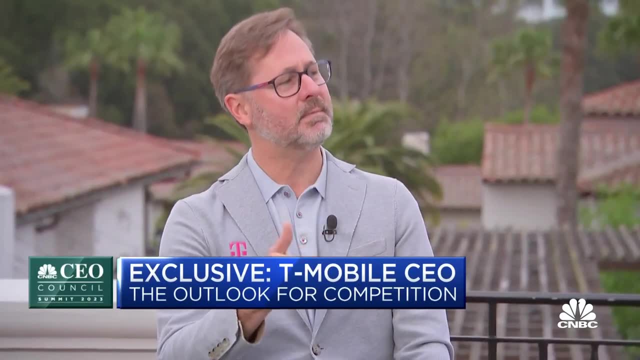 I mean we have more 5G landmass covered than AT&T and Verizon combined, And customers know that. now You know, and you see it in our credit- Our prime credit reached an all-time high in Q1 as a percent of our base. 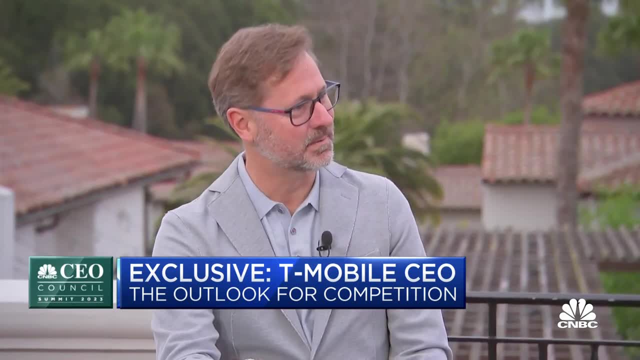 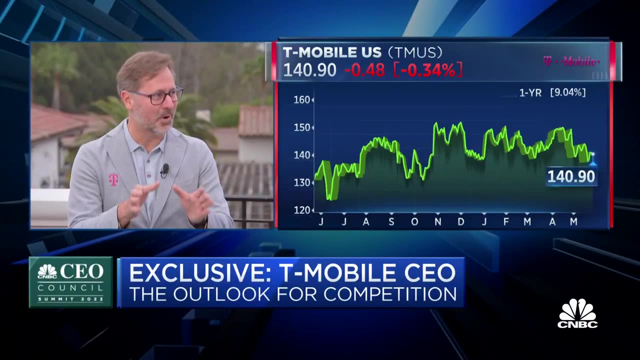 And our customers outperformed AT&T and Verizon customers in terms of bad debt. I mean, think about that. T-Mobile customers, including the former Sprint customers, pay their bills more reliably than AT&T or Verizon customers. That shows you the kind of people that are now choosing T-Mobile.